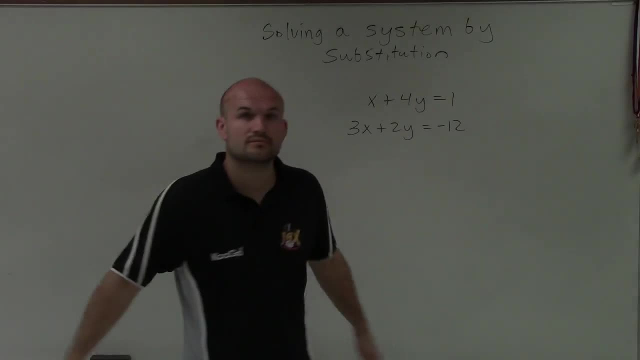 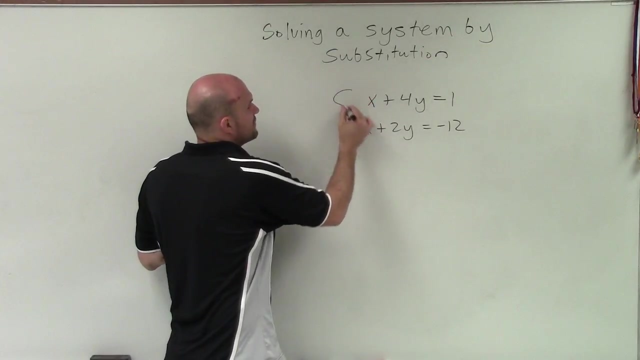 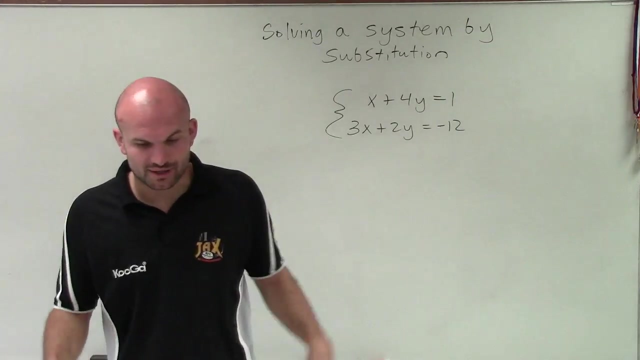 Well, so what I have here is x plus 4y equals 1, and 3x plus 2y equals negative 12.. Now, this is a good problem to look at substitution And when solving this by substitution. all I want to do is I want to look at what variable is going to be the easiest I can isolate or 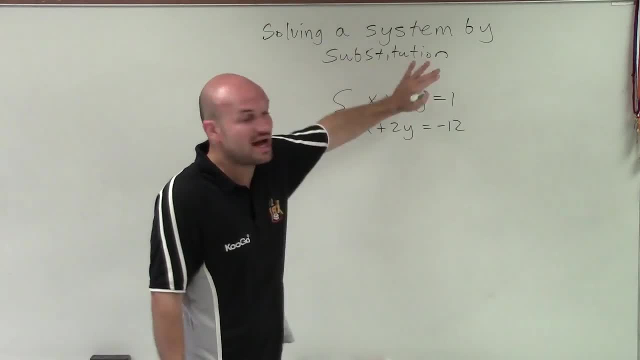 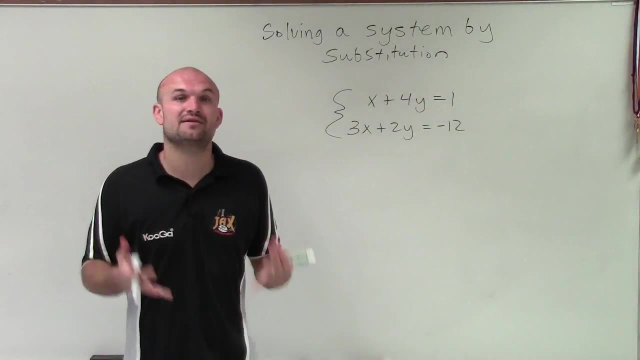 if one's already isolated. But I look at this and I notice that I do not have a variable: x or y, that's all by itself, right, That's on one side of the equation, all by itself. So what I need to do is I need to isolate that variable. Now we can pick any variable. 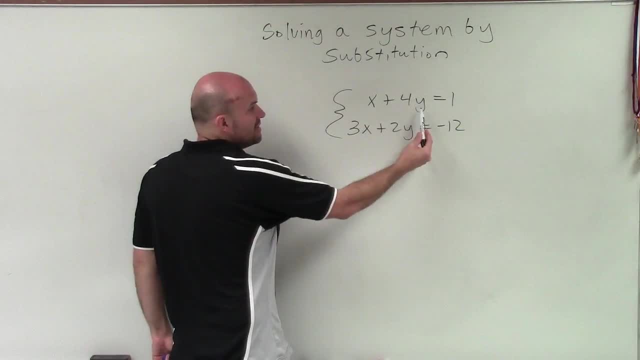 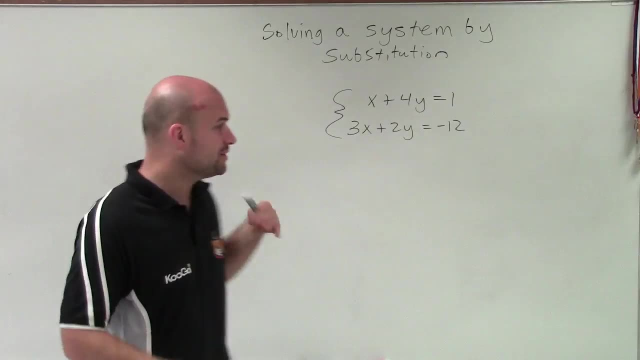 we want to isolate. I could solve for this x, I could solve for this y, I could isolate this y, isolate this x. But some of them are going to be easier than others. So when looking at an equation that I want to use substitution, I want to look for the variable that's going. 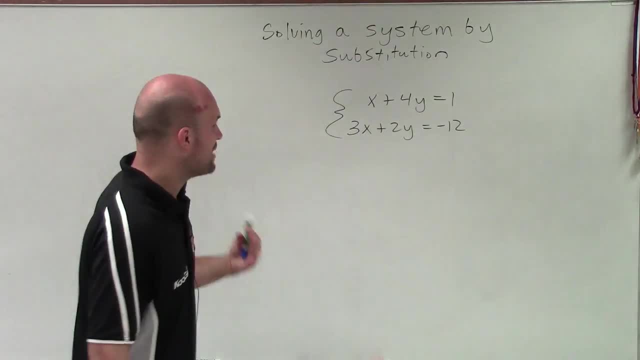 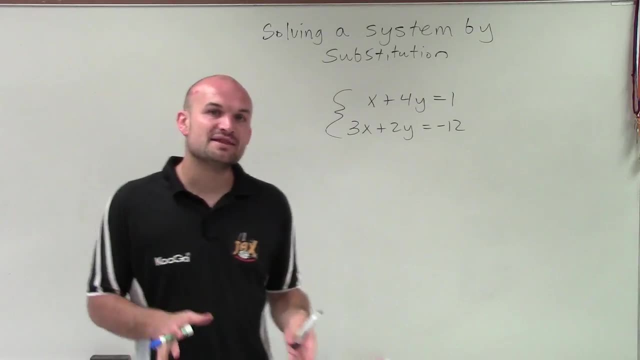 to be the easiest right. Why make things harder than they have to be? So I want to look for the variable that's going to be easiest to isolate. So what I like to do when I'm telling my students is find the variable that has a coefficient of 1 or negative 1, and that's the variable. 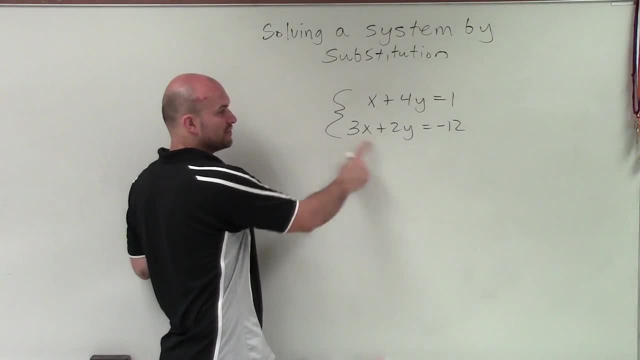 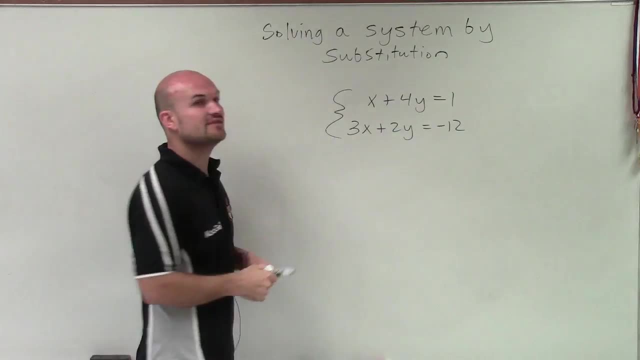 you want to isolate. Well, this x has a coefficient of 3.. This one has a coefficient of 2.. This variable has a coefficient of 4.. And this one has a coefficient of 1.. So, therefore, that's the variable that I'm going to want to isolate. So, to isolate it, what that means. 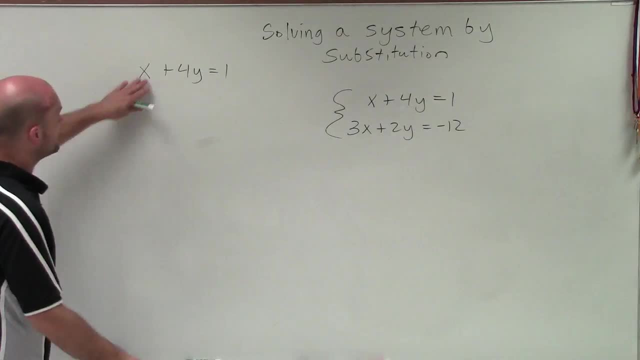 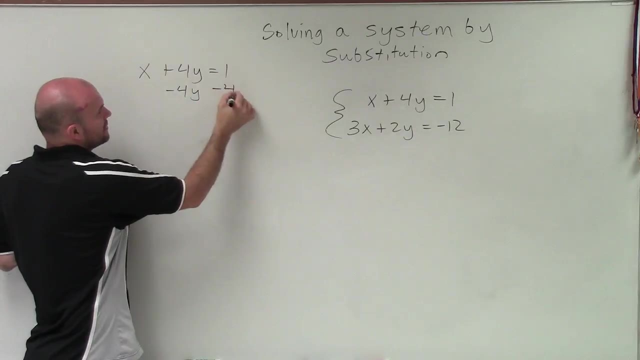 again is just to solve for that variable to get it all by itself. So to get x by itself, I'm going to write negative 4y, So I'm going to subtract 4y on both sides, So I have x equals 1 minus 4y, And a lot of times we like to write the variable in front, So I 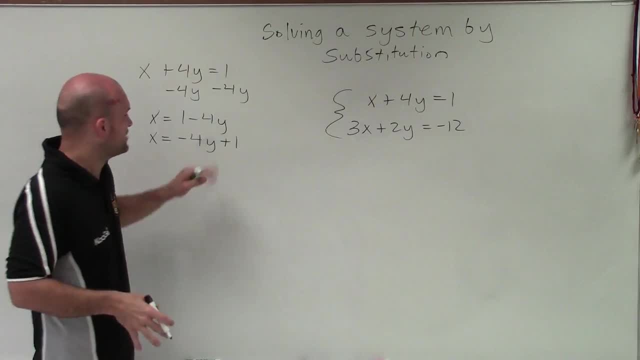 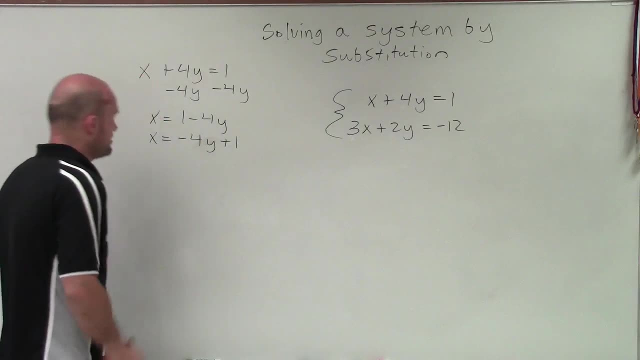 can write negative 4y plus 1.. But you don't have to. This is just a. in mathematics, we kind of like to always have the variable in front of our constant, But you don't have to change it at the end. So, therefore, what I'm going to do is I'm going to replace x. 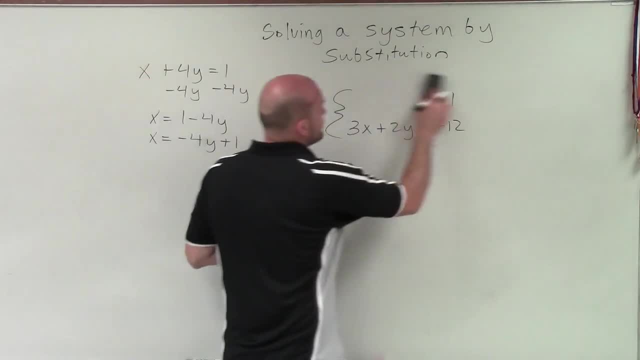 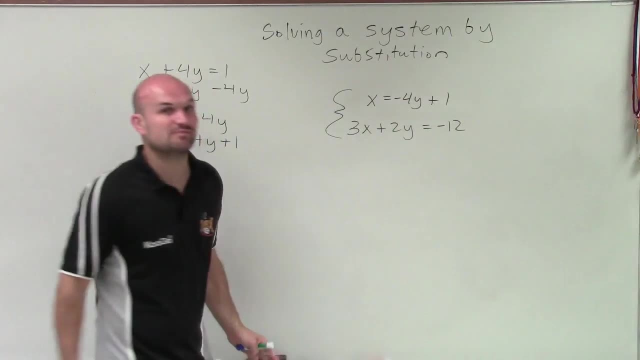 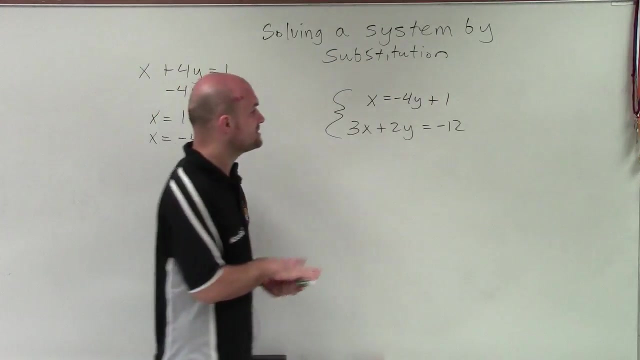 equals negative 4y in for this equation. It's the exact same equation, It's just written with the x now isolated. And the reason why we want to have this x isolated- because now we know the value of our variable x- is the expression negative 4y plus 1.. So when applying substitution, 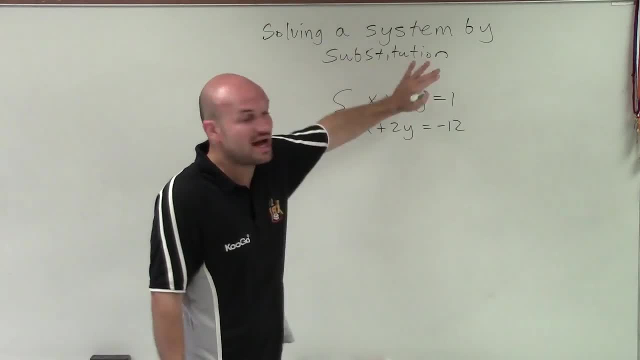 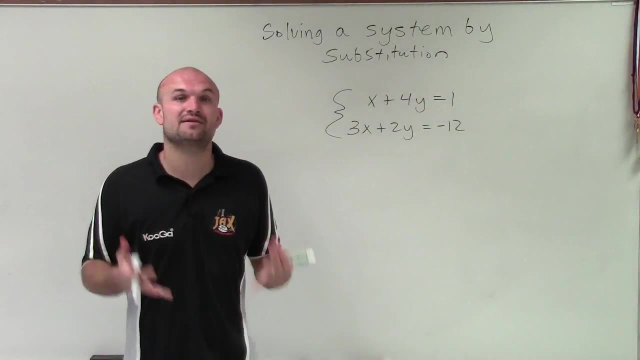 if one's already isolated. But I look at this and I notice that I do not have a variable: x or y, that's all by itself, right, That's on one side of the equation, all by itself. So what I need to do is I need to isolate that variable. Now we can pick any variable. 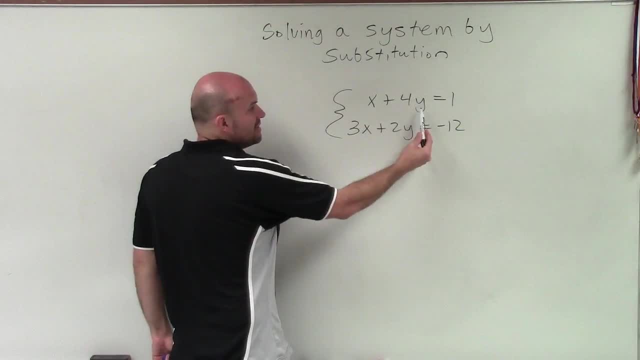 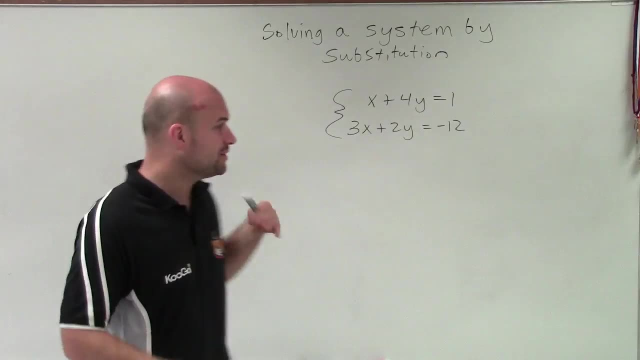 we want to isolate. I could solve for this x, I could solve for this y, I could isolate this y, isolate this x. But some of them are going to be easier than others. So when looking at an equation that I want to use substitution, I want to look for the variable that's going. 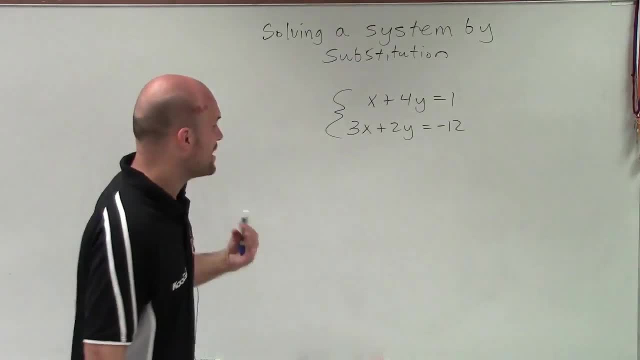 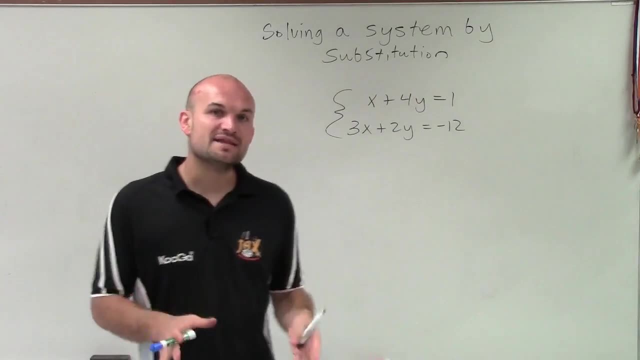 to be the easiest right. Why make things harder than they have to be? So I want to look for the variable that's going to be easiest to isolate. So what I like to do when I'm telling my students is find the variable that has a coefficient of 1 or negative 1, and that's the variable. 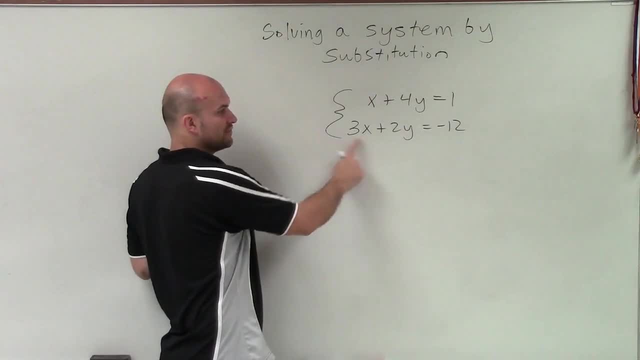 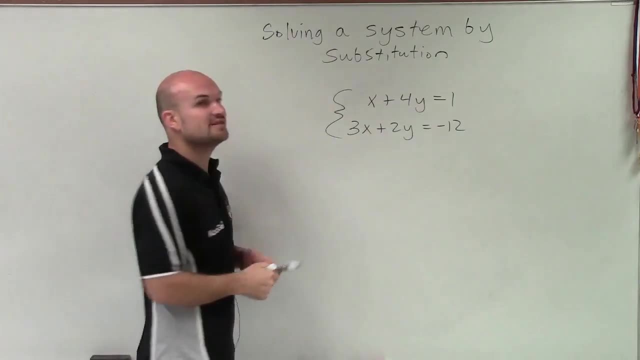 you want an isolate. Well, this x has a coefficient of 3, this one has a coefficient of 2, this variable has a coefficient of 4, and this one has a coefficient of 1.. So, therefore, that's the variable that I'm going to want to isolate. So, to isolate it, what that means. 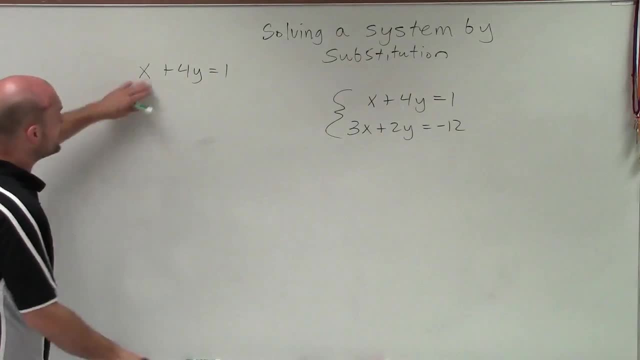 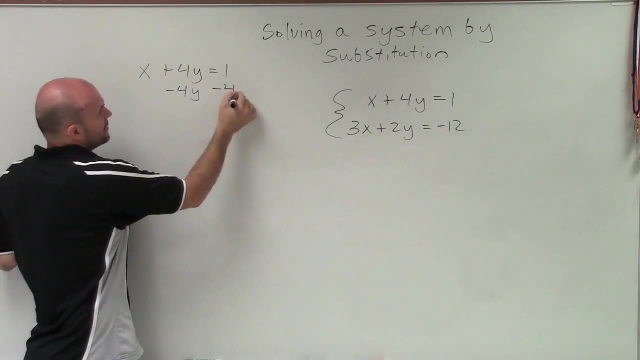 again is just to solve for that variable to get it all by itself. So to get x by itself, I need to undo what's happening to the variable. It's being added by itself And what? I'm going 4y. So I'm going to subtract 4y on both sides So I have x equals 1 minus 4y, And a lot of times. 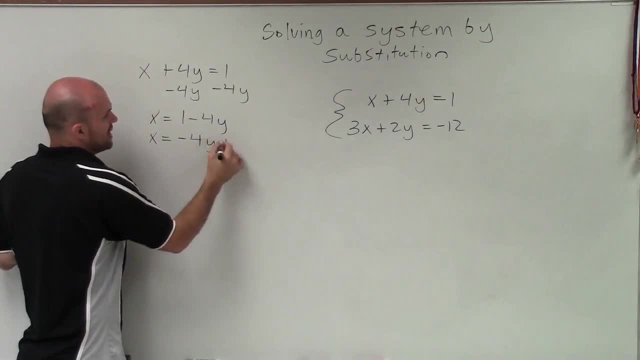 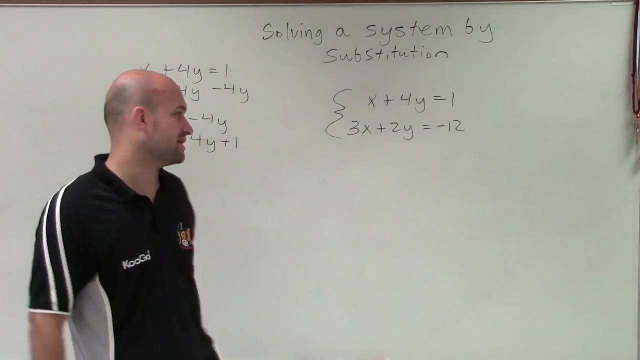 we like to write the variable in front, So I can write negative 4y plus 1.. But you don't have to. This is just a. in mathematics we kind of like to always have the variable in front of our constant, But you don't have to change it at the end. So therefore, what I'm going to do is I'm 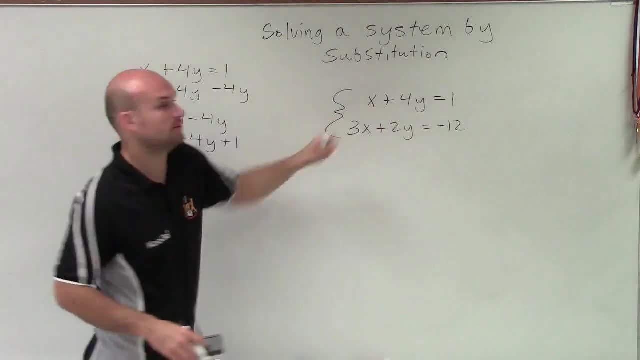 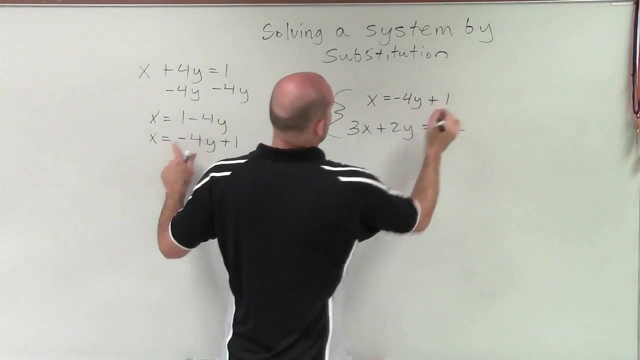 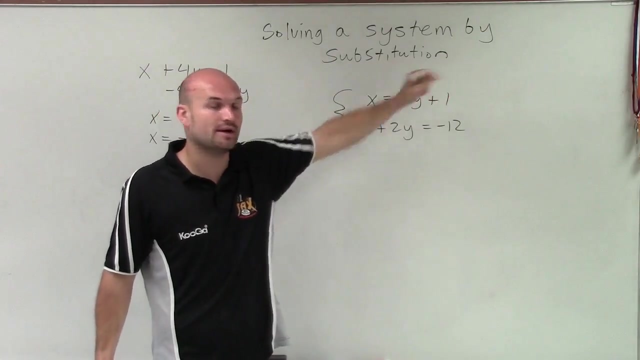 going to replace x equals negative 4y in for this equation. It's the exact same equation, It's just written with the x now isolated. And the reason why we want to have this x isolated- because now we know the value of our variable x- is the expression negative 4y plus 1.. So when applying 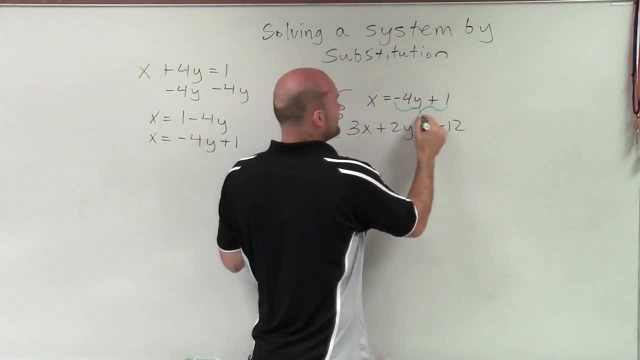 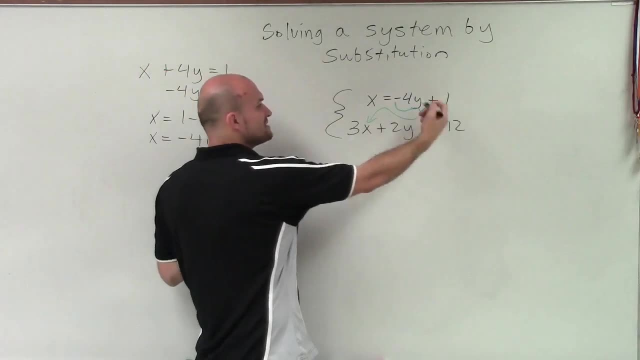 substitution. I can apply this value in for x into our other variable in the other equation. So what that looks like. so now, if I rewrite this by substituting in the value of x for the variable in the other equation, it's going to be 3 times. 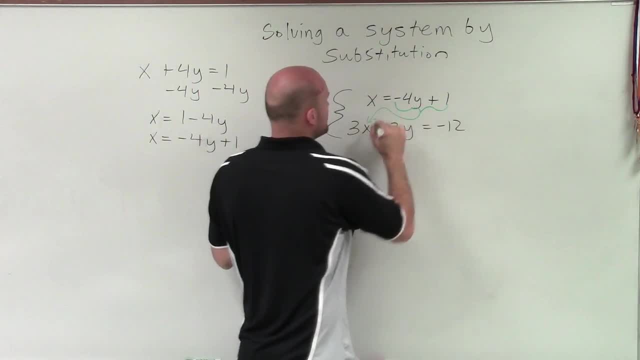 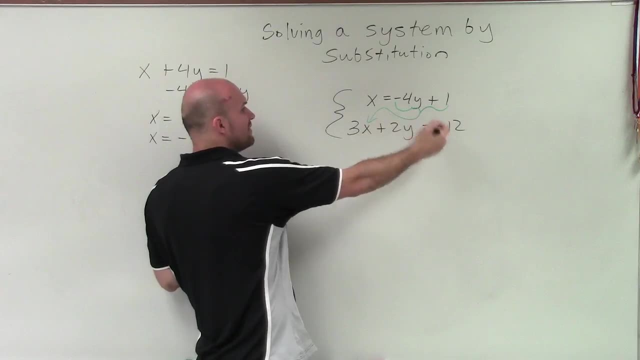 I can apply this value in for x into our other variable in the other equation. So what that looks like. so now, if I rewrite this by substituting in the value of x for the variable in the other equation, it's going to be three times, not just x. 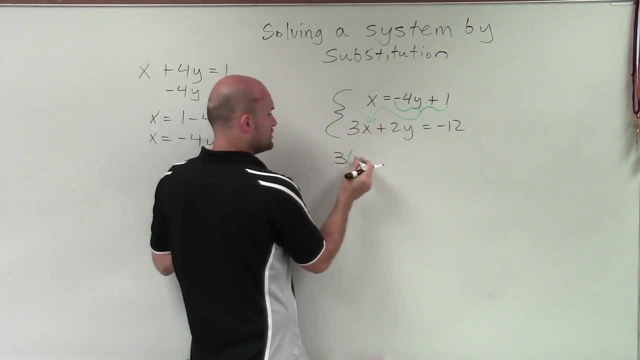 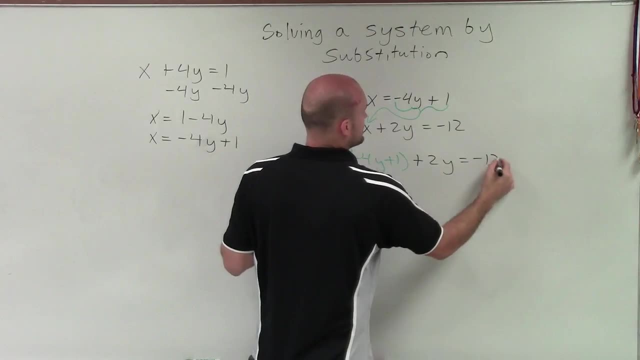 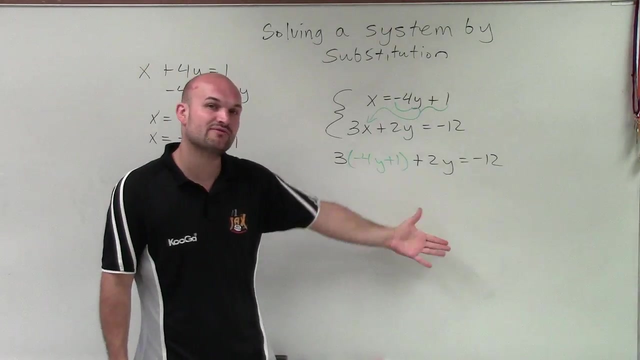 But now the value of x, which we achieved from our other equation, which is negative: 4y plus 1 plus 2y equals negative 12.. And again, the reason why this is so important is because now I created an equation with only one variable. 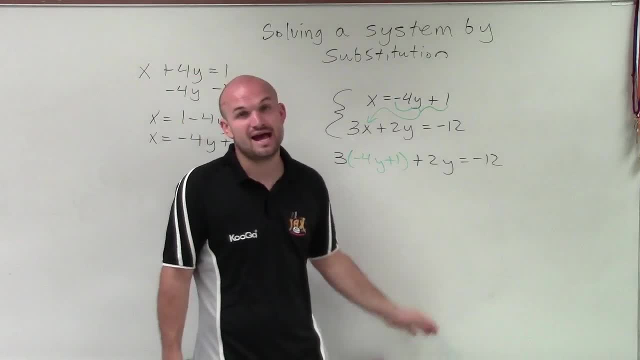 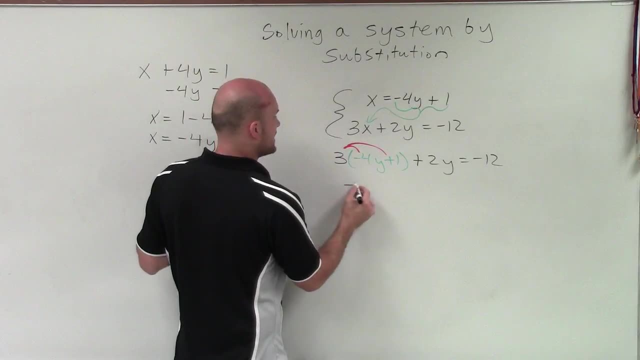 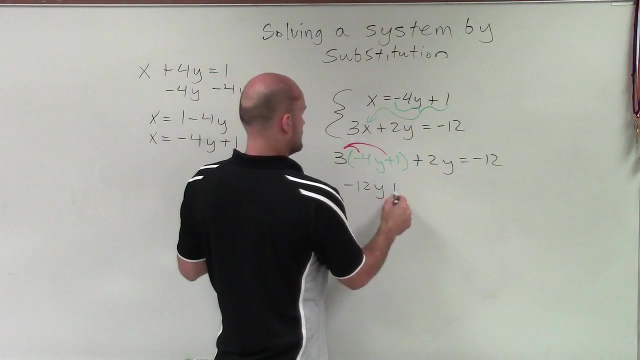 And I can solve for my variable y when I only have that one variable in the equation. So before I do that, though, I need to simplify this a little bit. So I apply distributive property, So I have a negative 12y plus 3 plus 2y equals negative 12.. 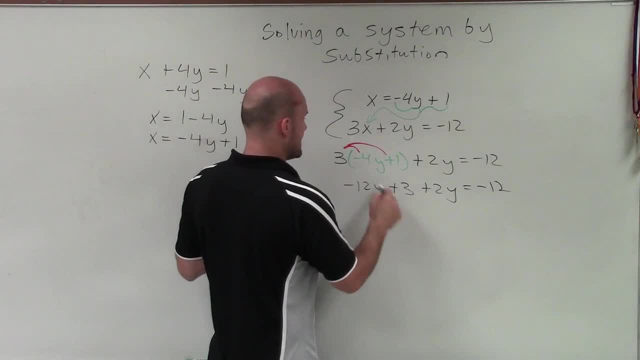 Then I combine my like terms, So therefore this becomes a negative 10.. I combine my two y values. Those are like terms, So it becomes a negative 10y plus 3 equals negative 12. Then I subtract 3 on both sides. 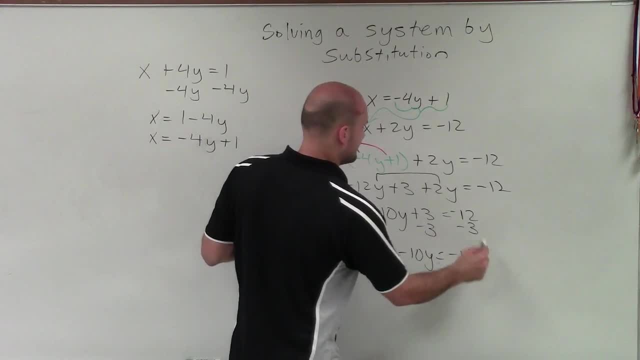 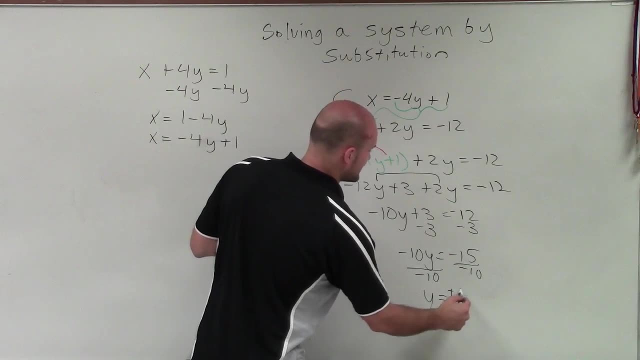 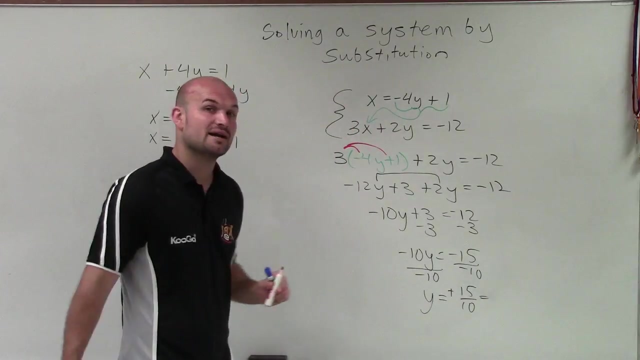 And I get a negative 10y equals a negative 15.. Well, I divide by negative 10.. And I get: y equals a positive 15 over 10.. Now, remember, I can simplify this right. I can simplify this by dividing the top and bottom, the numerator and the denominator by 5.. 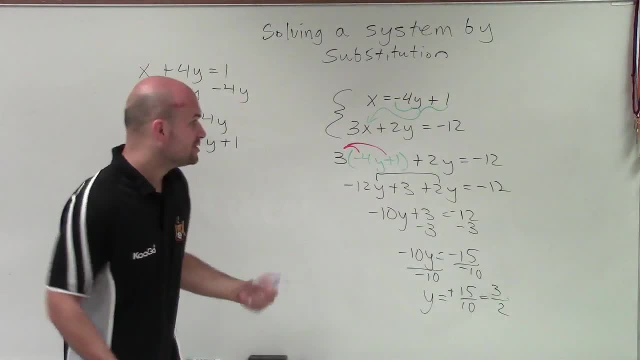 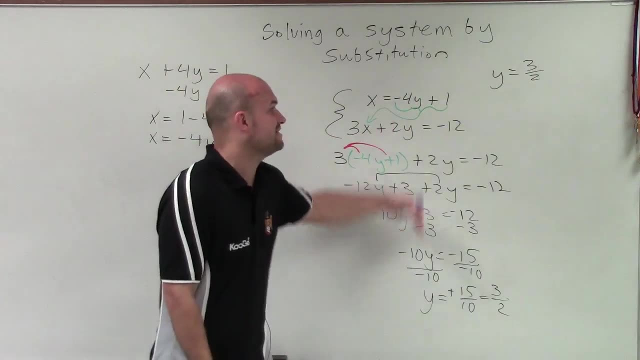 I can resubstitute this in as 3 halves, So the value of y that makes both equations true is going to be 3 halves. Now what I need to do Is find the value of x that's going to make this true. 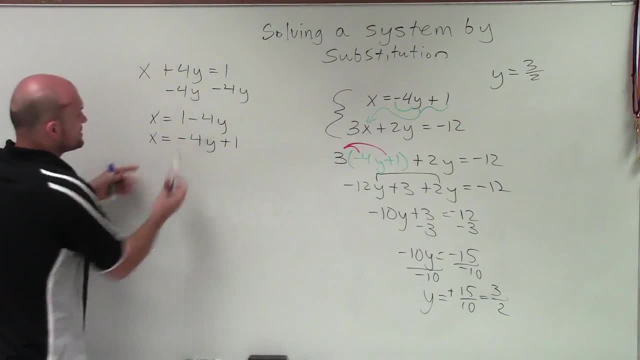 And what's nice about using the substitution method Is when I spend all this time isolating my variable. If I know now the value of y To find the value of x, all I need to do is plug it back into this equation. 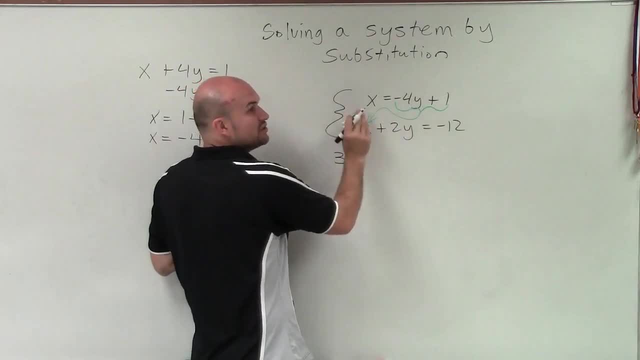 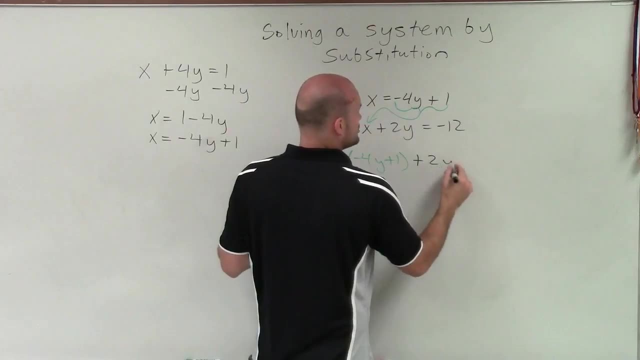 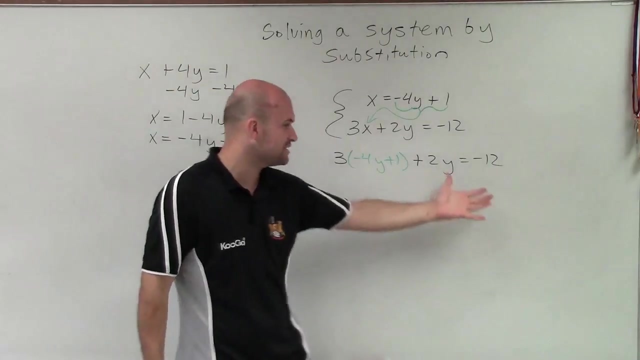 not just x, but now the value of x which we achieve from our other equation, which is negative: 4y plus 1. Plus 2y equals negative 12.. And again, the reason why this is so important is because now I created an equation with only one variable And I can solve for my variable y when I only have 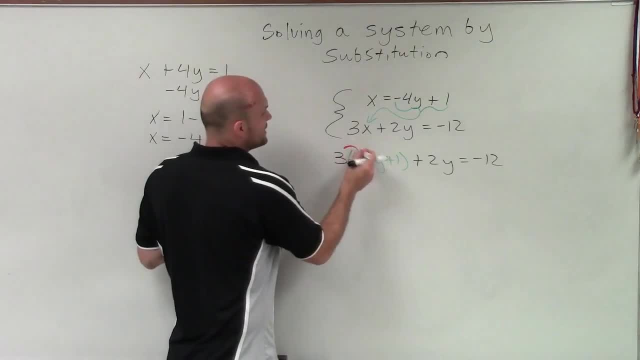 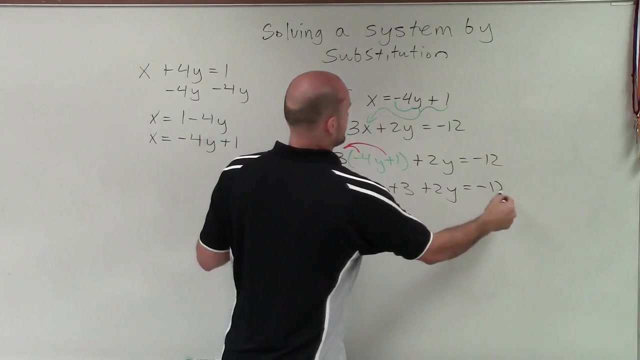 that one variable in the equation. So before I do that- though, I need to simplify this a little bit. So I apply distributive property, So I have a negative 12y plus 3 plus 2y equals negative 12.. Then I combine my like terms. So therefore, 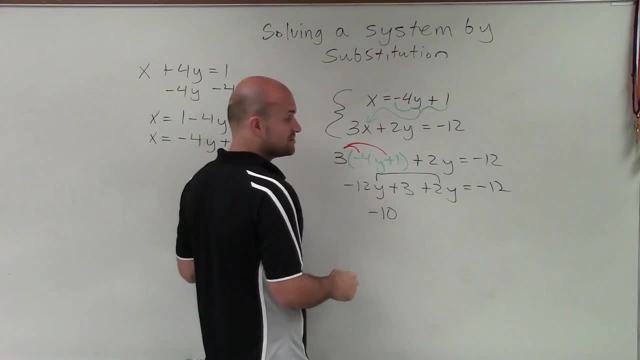 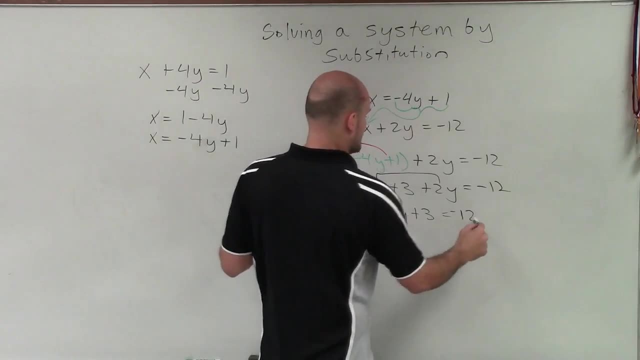 this becomes a negative 10.. I combine my two y values- Those are like terms, So it becomes a negative 10y plus 3 equals negative 12.. Then I subtract 3 on both sides and I get a negative 10y. 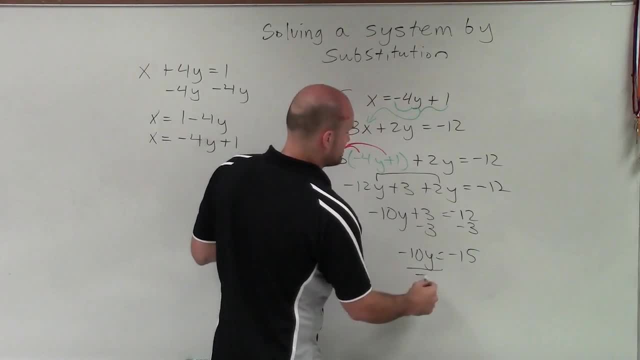 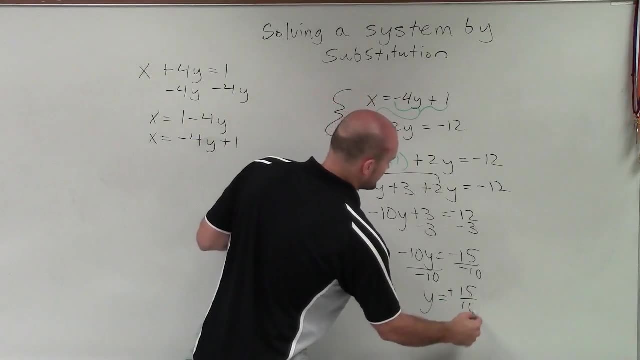 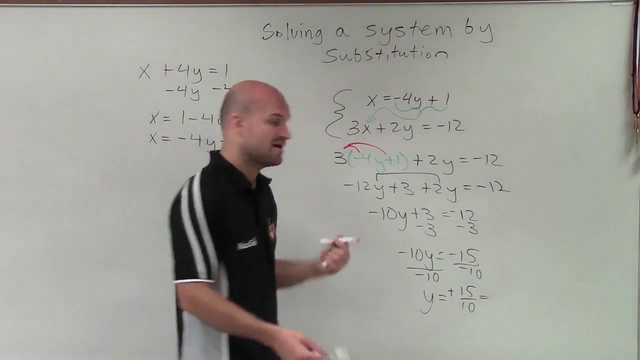 equals a negative 15.. Well, I divide by negative 10. And I get: y equals a positive 15 over 10.. Now, remember, I can simplify this. I can simplify this by dividing the top and bottom, the numerator and the denominator by 5.. 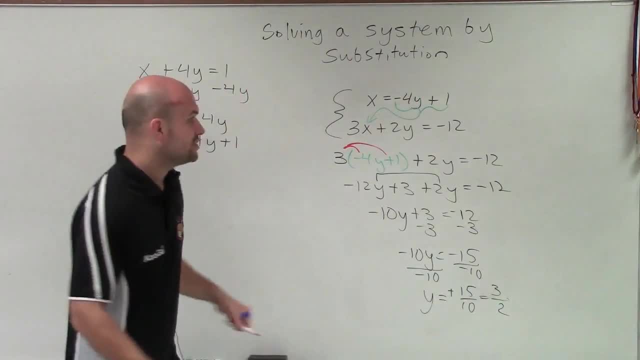 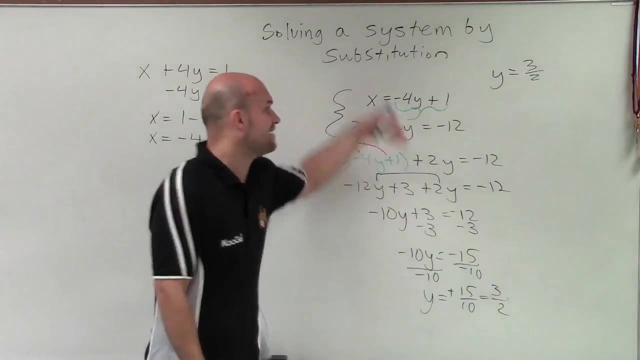 I can resubstitute this in as 3 halves, So the value of y that makes both equations true is going to be 3 halves. Now what I need to do is find the value of x that's going to make this true. And what's nice about using the substitution method? 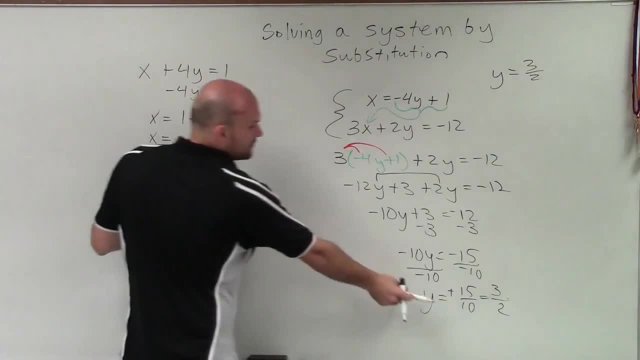 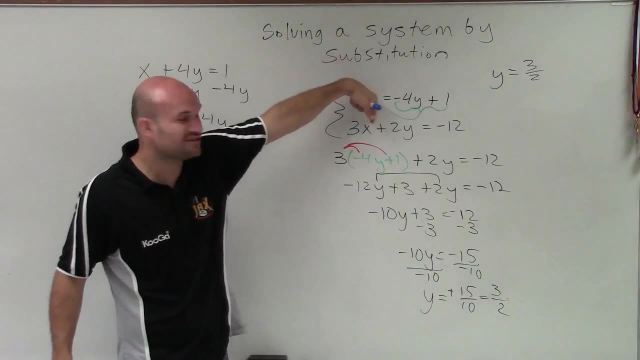 is when I spend all this time isolating my variable. if I know now the value of y, to find the value of x, all I need to do is plug it back into this equation. You can plug it into this equation, but you're having a lot more work. 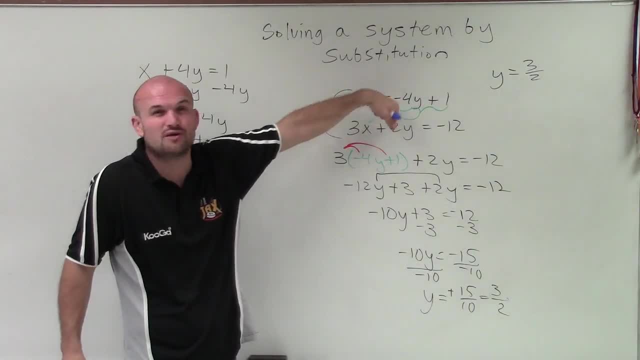 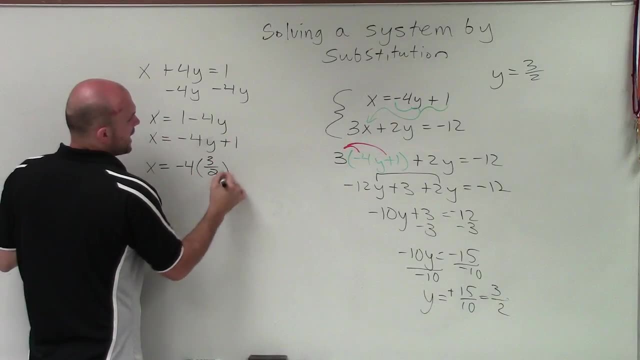 You can plug it into this equation, But you're having a lot more work having to solve for your variable. So when I plug it back into this equation, I have x equals negative 4 times 3, halves plus 1.. Now remember, when multiplying a whole number times a fraction, 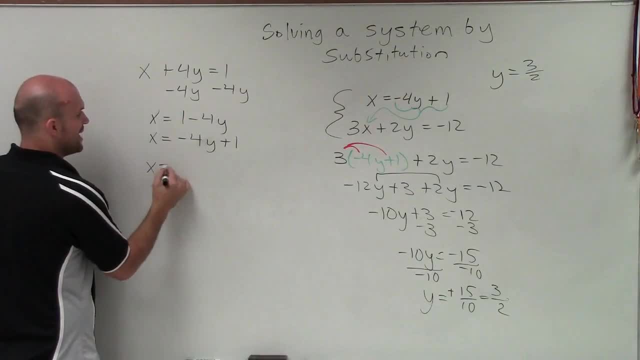 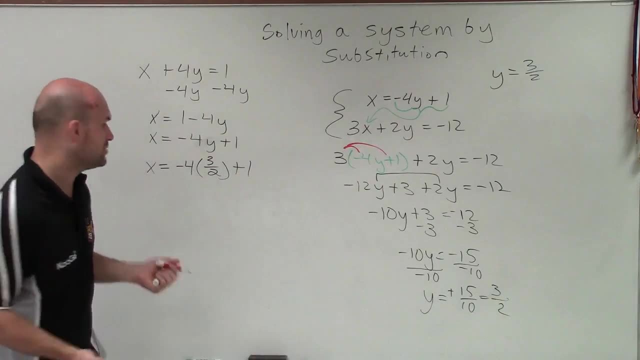 having to solve for your variable. So when I plug it back into this equation, I have: x equals negative 4 times 3, halves plus 1.. Now remember: when multiplying a whole number times a fraction, I can make this into a fraction.